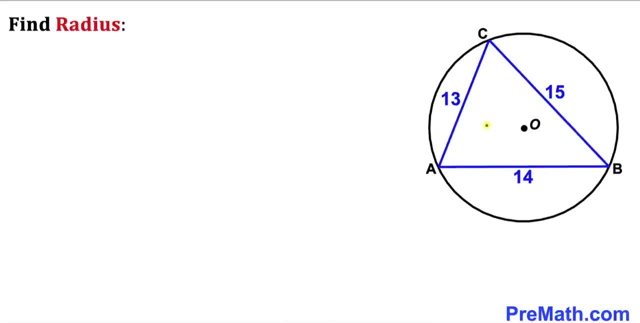 And here's our very first step. Let's go ahead and draw some auxiliary lines to solve this problem. Therefore, I have dropped this perpendicular CD on this line AB. Let's assume that this segment is a line AB And this segment AD is X units and this perpendicular CD is lowercase h. 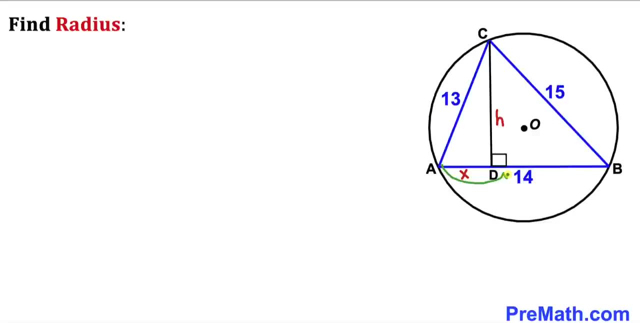 And now let's make an observation. We know that this whole AB chord is 14 and this segment AD is X. So therefore, this segment BD is going to be 14 minus X. And here's our first step. Let's go ahead and draw some auxiliary lines to solve this problem. Please don't forget to give a thumbs up and subscribe. Please keep in mind that this figure may not be 100% true to the scale. Let's go ahead and draw some auxiliary lines to solve this problem. Please keep in mind that this figure may not be 100% true to the scale. 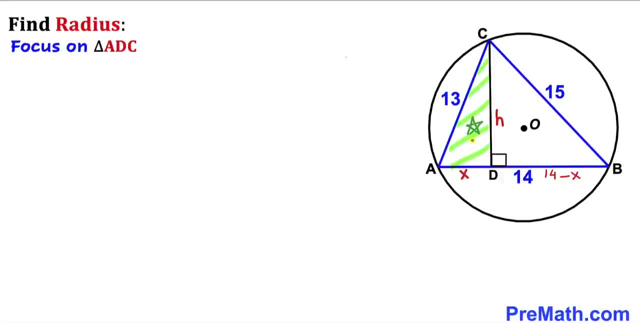 And here's our first step. Let's focus on this right triangle, ADC, And we are going to use the Pythagorean theorem. And here's our Pythagorean theorem: A square plus B square equal to C square. Let me go ahead and call this longest leg as our side C. I'm going to call this side A and this side lowercase b. 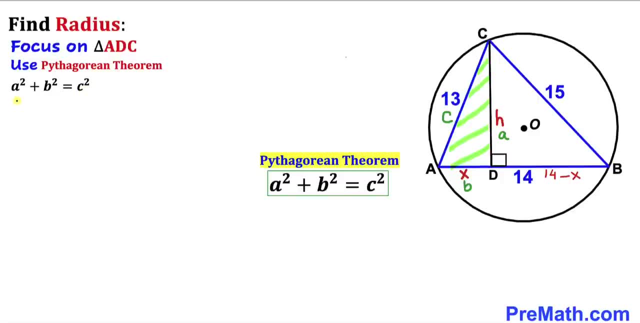 So let's go ahead and fill in the blanks in this Pythagorean formula. A, in our case, is h, So it's going to become h. square plus b is X. It's become h square plus b is X. x square equal to 13 square. and now 13 square on the right hand side is 169, as you can see in this. 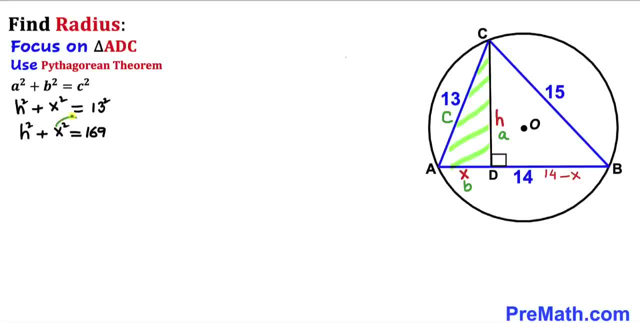 next step now let's go ahead and move this x square on the right hand side, so therefore, we are going to have h square equal to 169 minus x square. let me go ahead and call this our equation number one. and here's our next step. let's focus now on this. another right triangle: b, d, c and we: 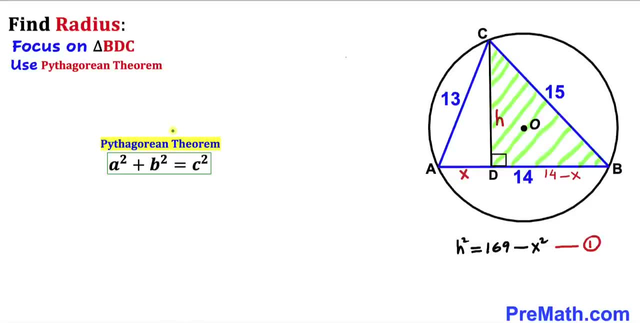 are going to use the pythagorean theorem once again. and here's our pythagorean theorem. once again, let me label this longest leg as our side c. i'm going to call this side lowercase a and this side lowercase b. now let's go ahead and fill in the blanks in this pythagorean formula a, in our 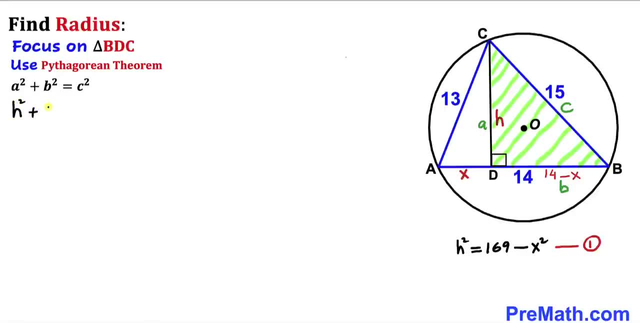 case is h, so this become h square plus b. in our case is 14 minus x whole square equal to c. in our case is 15 whole square. now let's go ahead and simplify. so we got h square plus and now let's recall this famous identity: a minus b. 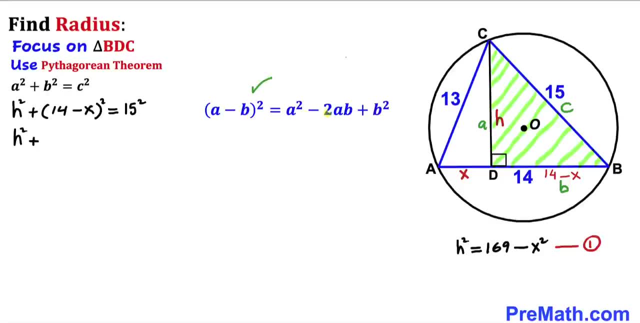 whole square could be written as a square minus 2, a, b plus b square. now let's go ahead and apply on this binomial. so therefore, this could be written as 196 minus 28 x plus x square equal to 15. square is 225. and now let's go ahead and move all these. 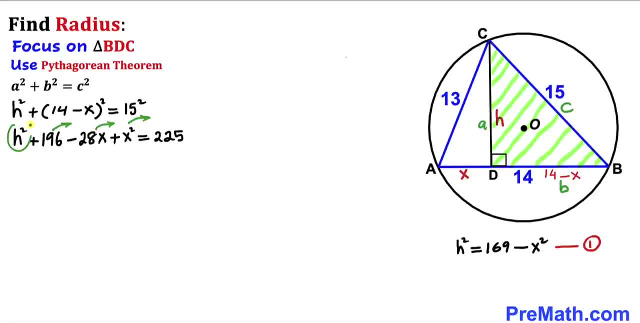 terms to the right hand side to isolate h square. so therefore we got h square equal to 225 minus 196 plus 28 x minus x square. now let's go ahead and combine these like terms. so therefore we are going to have a. let me go ahead and call this our equation number two. and here we got equation one. 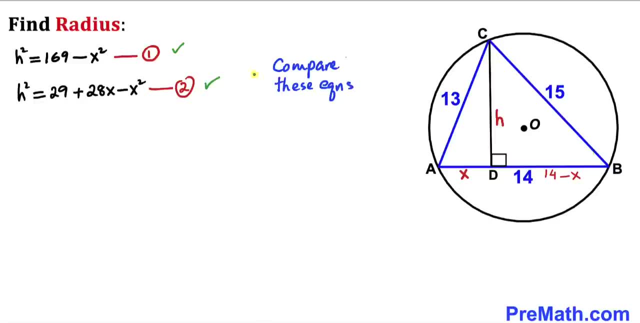 and equation two. let's go ahead and compare these two equations, since the left hand sides are same, so therefore we can equate the right hand sides as well. so therefore i can write: 29 plus 28 x minus x square is going to be equal to 169 minus x square. 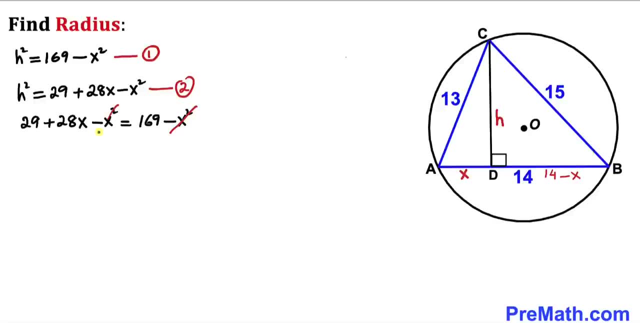 and now we can see this negative x square and this negative x square. they are gone. now let's go ahead and move this 29 on the other side. so therefore, we are ended up with 28 x equal to 169 minus 29. now let's go ahead and divide both sides by 28. this is gone, so therefore. 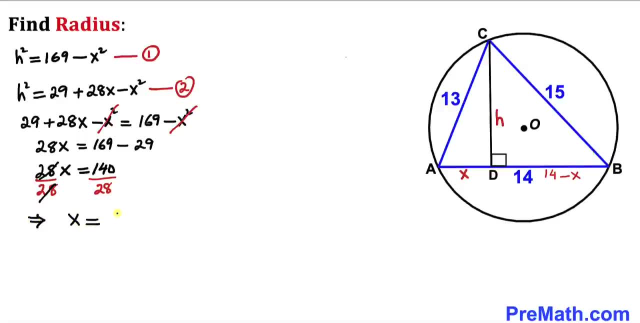 our x value turns out to be 5. so therefore, x value turns out to be 5 units. now let's go ahead and calculate the value of this h by plugging in this x value in this equation 1. and here's our equation 1. let me go ahead and replace x by 5, so therefore, 5 square is going to become 25. 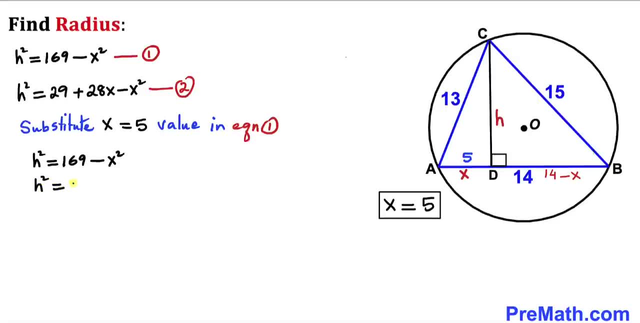 so, therefore, we got h square equal to 169 minus 25 and in this next step, 169 minus 25 is going to give us 144. now let's go ahead and undo this square by taking a square root on both sides. so therefore, our h value. 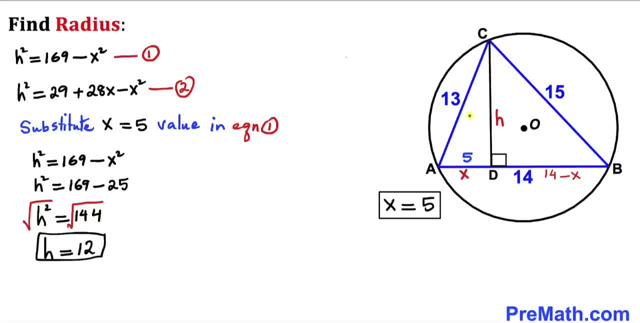 turns out to be positive: 12. so therefore our perpendicular h value turns out to be 12, and also we could have found this h value by using the pythagorean triplets 5, 12 and 13, since 5 and 13 are given. so therefore, unknown value is going to be 12 on this side. and here's our next step. i have 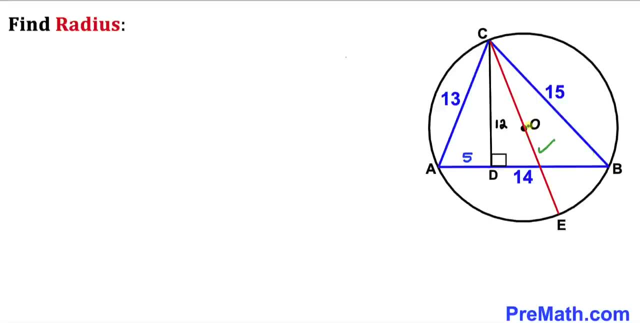 drawn this diameter ce that passes through this center o, and now our task is to calculate the value of this diameter c in order to find the radius of this circle. and here i have connected this point e with this point b, so we got this chord e, b, and now let's recall the Thales theorem, according to 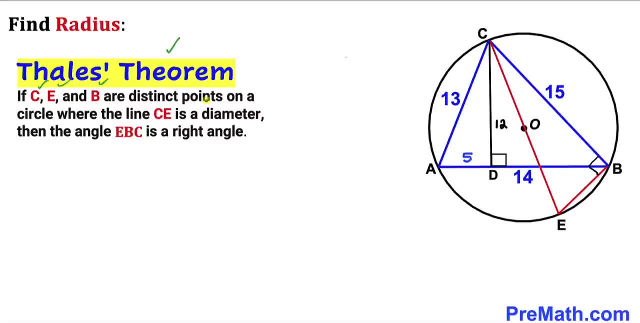 this theorem: if c, e and b are our three distinct points on the circle with the line is a diameter, then the angle e, b, c is a right angle. as you can see in our this diagram we got these points: c, e and b are our three distinct points and c, e is the diameter, then no wonder. 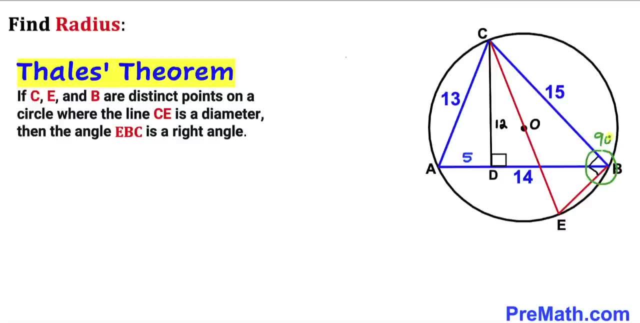 this angle- e, b, c- is going to be 90 degree angle. and here's our next step. let's recall inscribed angles theorem. according to this theorem, inscribed angles that intercept the same arc are congruent. so therefore, this angle, this one, c, a, b, this angle intercepts this green arc. let me call this angle. 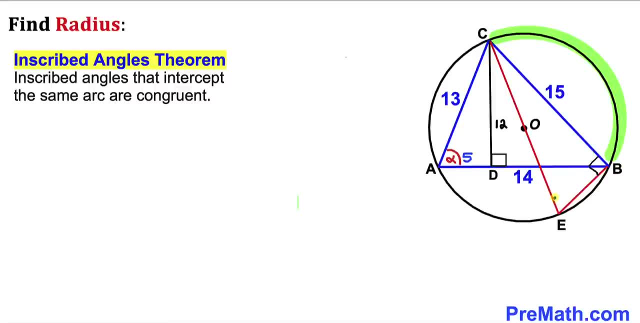 alpha, and we can see that this angle c e b also intercepts the very same green arc. so, therefore, this angle c e b is going to be 90 degree angle. and here's our next step. let's recall, therefore, this angle is also going to be alpha. so therefore, we conclude that these are two angles. 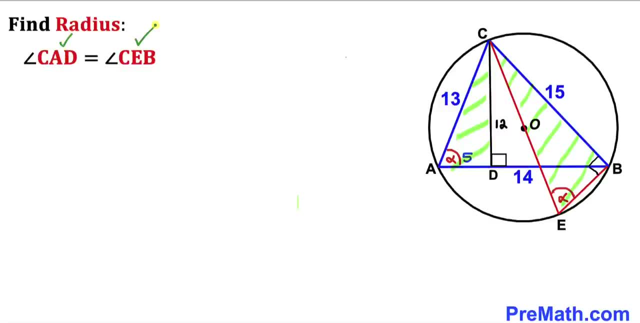 c, a, d and the other angle, c, e, b, are congruent. so therefore we conclude that these are two triangles: e, b, c and the other triangle, a, d, c are similar triangles according to angle angle similarity theorem. since this angle is 90 degrees, this angle is alpha. 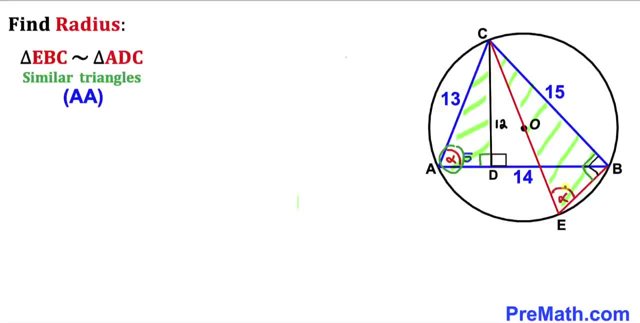 likewise over here. this angle is 90 degrees and this angle is alpha as well, so therefore we are going to have a proportion. let's go ahead and write down the ratio of this c e length and this length b c. so let me write down: the ratio of c e divided by b c is going to be equal to: 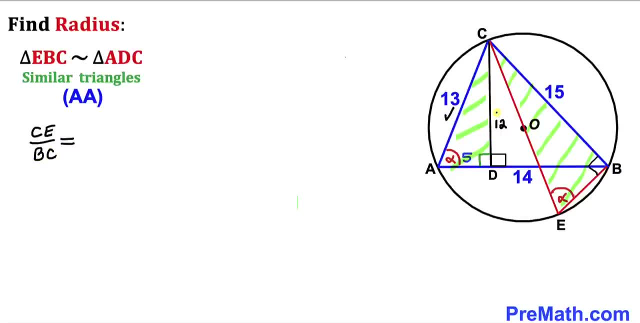 the ratio of a, c and b c. so we have this angle, which is 90 degrees, and this angle is alpha as well, and CD. Let me go ahead and write down AC divided by CD, And now our BC length is 15.. Our AC length: 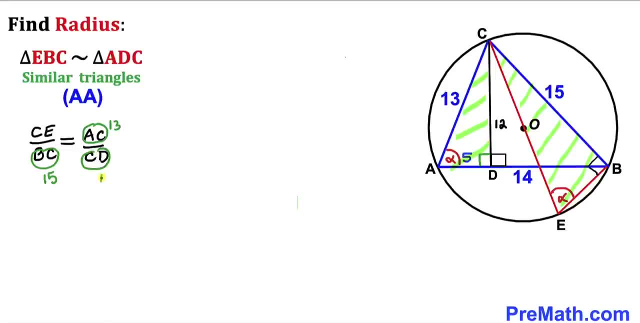 is 13.. And our CD length is 12.. So therefore, I can write: CE divided by 15 equal to 13 divided by 12.. Let's go ahead and multiply both sides by 15 to isolate CE. I'm going to multiply 15 on this. 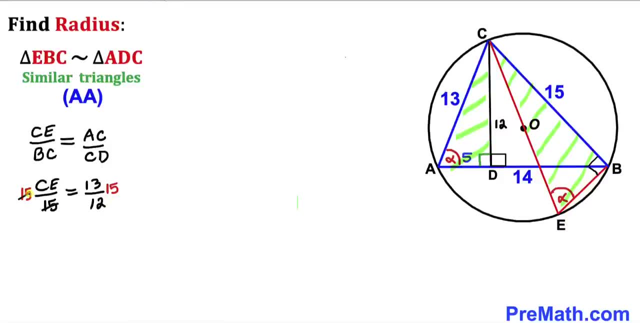 side as well. So we can see this: 15 and 15 is gone. So CE length turns out to be: and here 15 divided by 12 could be reduced to 5 divided by 4.. So therefore, this is going to become 65. 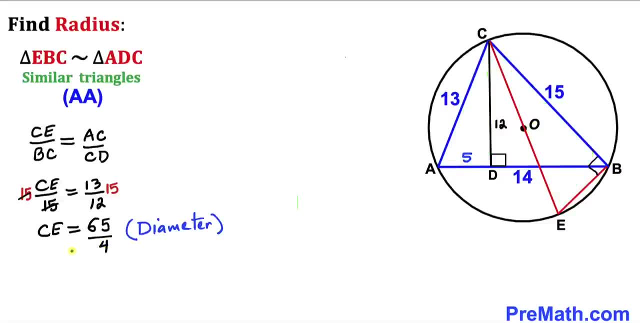 divided by 12.. So we can write down AC, divided by 12, equal to 13 divided by 12.. And now our BC length is 15.. So we can write down CE, divided by 12, equal to 13 divided by 12.. And now we can. 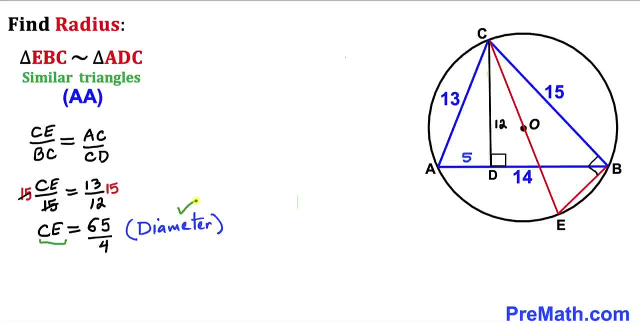 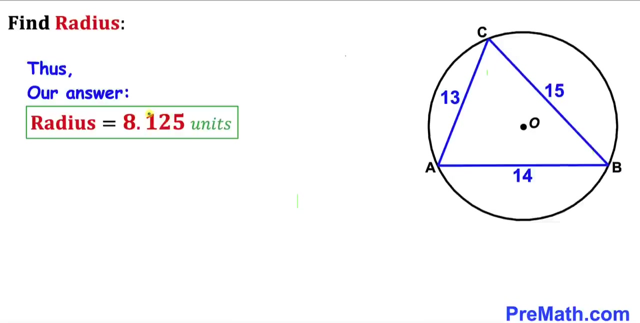 see that this CE is the diameter of this circle. So therefore, the radius of this circle is going to be half of this one. So that is going to be 65 divided by 8 units, And that would be equal to 8.125 units. So thus the radius of this given circle turns out to be 8.125.